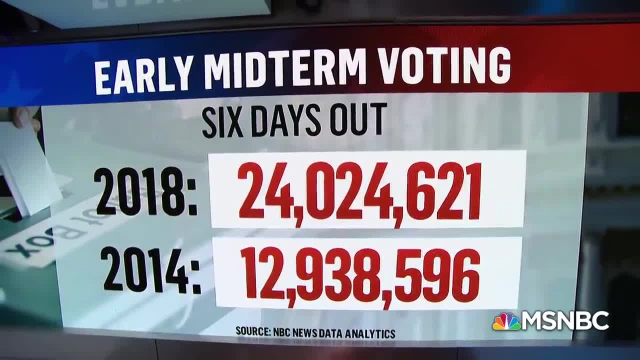 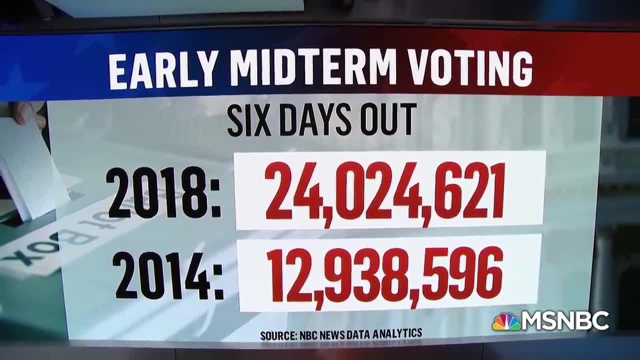 Voters are already coming out in droves to make their voices heard. As of Wednesday, according to NBC News analysis, more than 24 million early votes have been cast- almost double the number at the same time in the 2014 midterms. 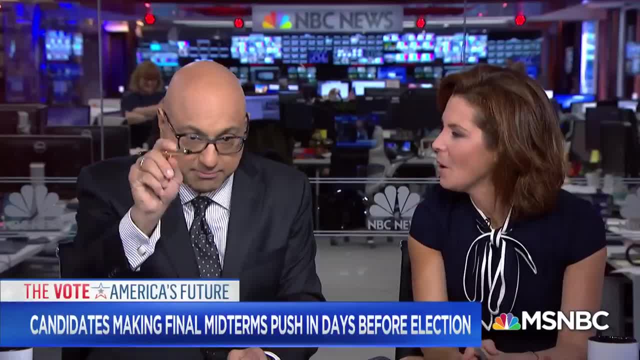 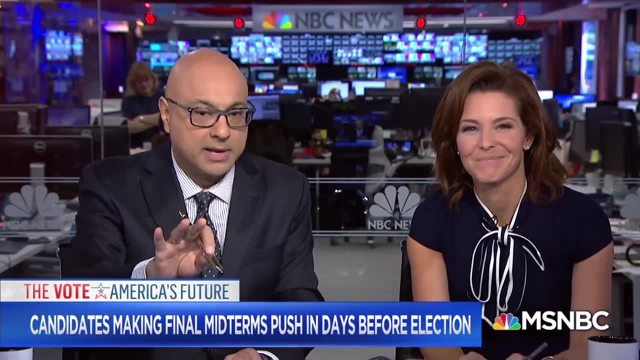 That's incredible. You said it yesterday. The greatest news you and I could have, That's it would be next Wednesday morning waking up to tell you Breaking news: Record numbers of people have voted. It's not the outcome, It's that you voted. 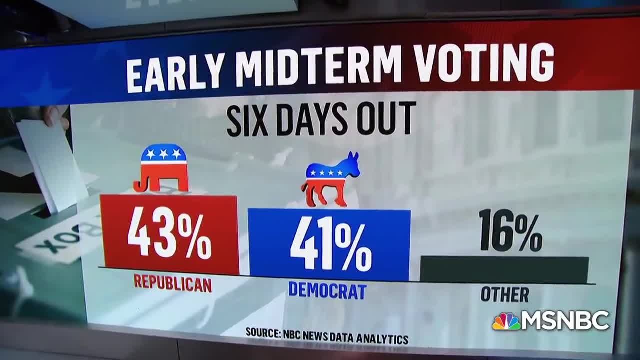 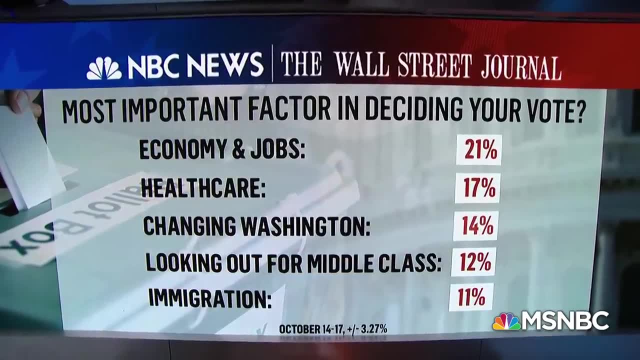 43% of people have voted. Casting early ballots are Republicans. 41% are Democrats. 16%. identify as other Some of the biggest issues affecting how people will vote first- and we talk about this all the time. It is not necessarily the hot-button issues that you hear candidates talking about. 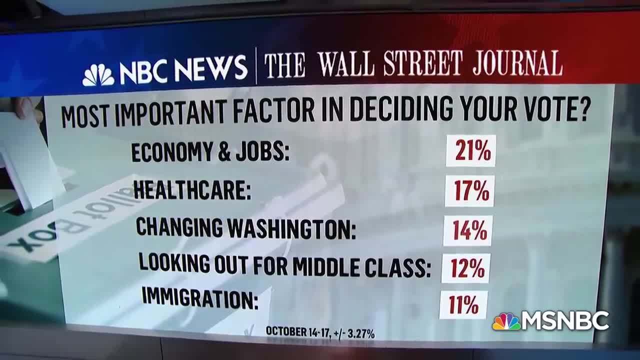 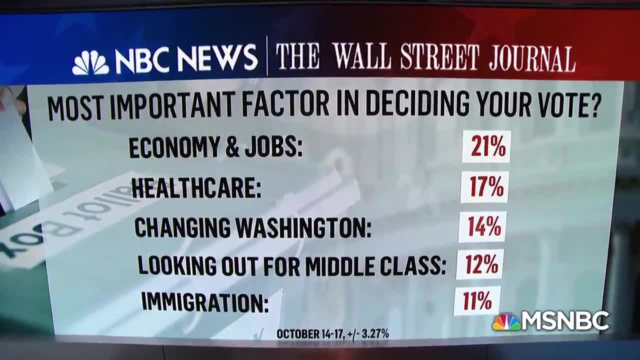 It's the economy, It's jobs. Second, it's health care. Third, changing how things work in Washington. We've heard that frustration with government leadership. Fourth, looking out for the middle class, Which is basically the same as economy and jobs and health care right. 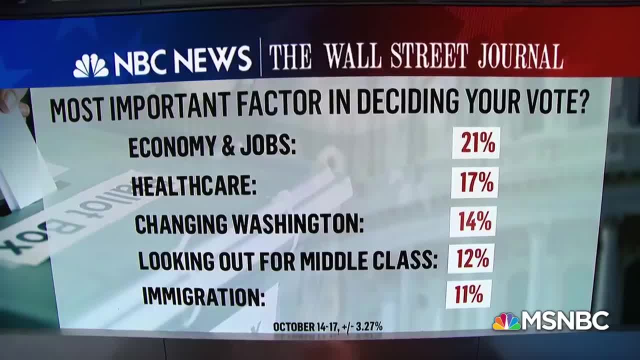 It's all tied in. When you talk about looking after the middle class, it's economics, Except here's your issue. You want to look out for the middle class. The president says we have a middle-class tax cut coming up. I say where? 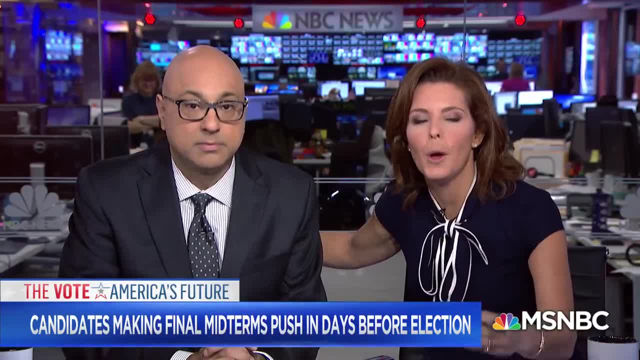 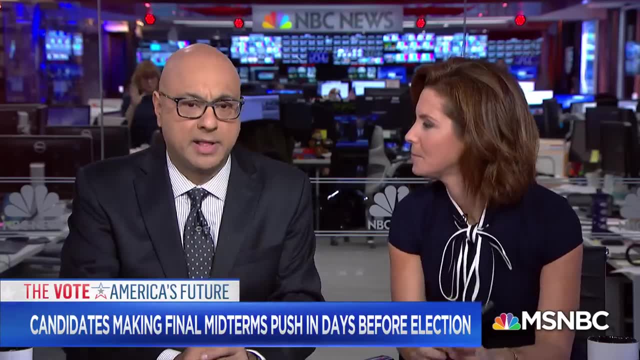 Not only is Congress not in session, how do you pay for it? The president has given Zippo zero zilch information of how he's going to do that Because, remember, I can talk about how we paid for the last tax cut. 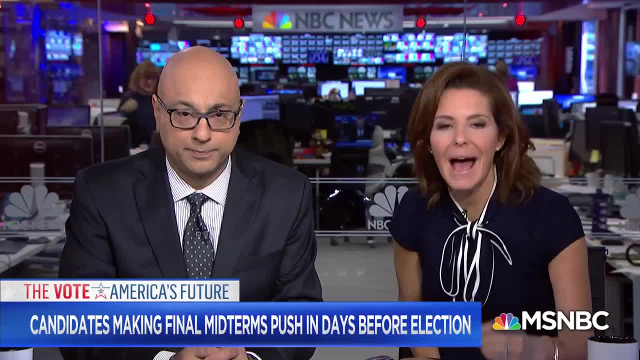 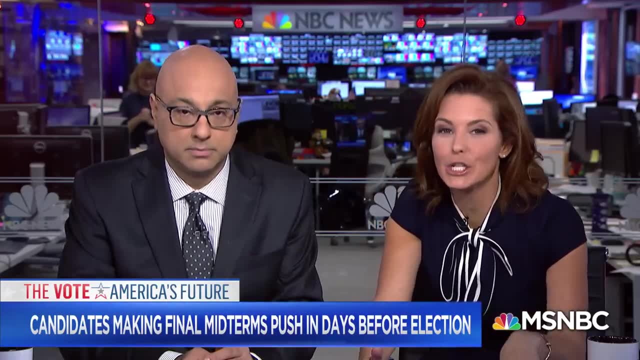 Maybe we can do it the same way, Stephanie, Don't be sassy. Okay, We gave a massive tax cut to corporate America. Now you could have given a tax cut to corporate America, a lesser one And an additional one, a separate one for the middle class. we didn't. 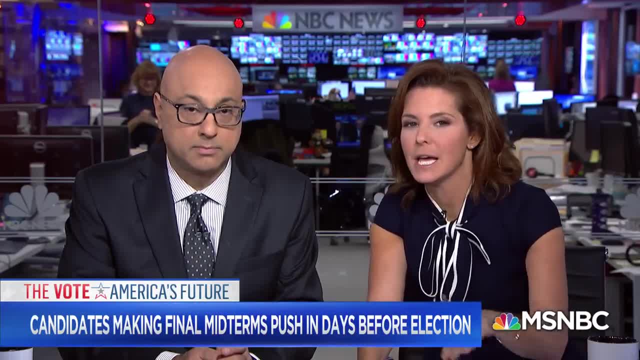 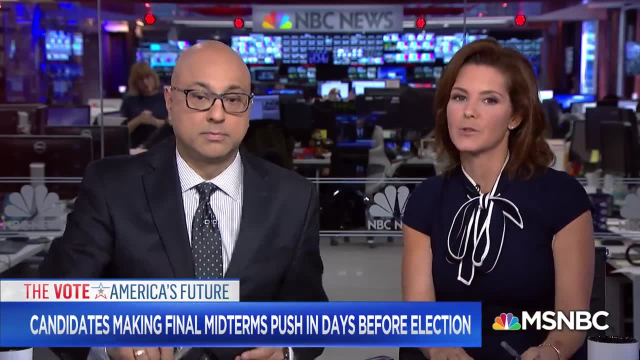 So now here we are with a tax cut that hasn't paid for itself, And the president is talking about a second one, And we're here to tell you there is no formula to pay for it. Fifth, it's President Trump's favorite one. 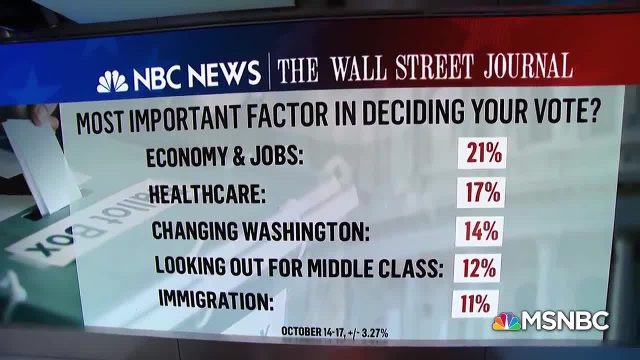 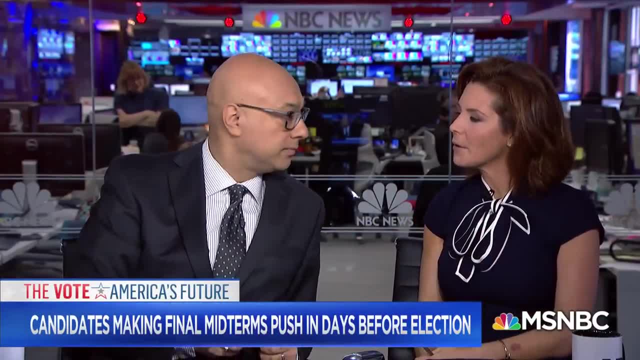 Right, it's the last one there. immigration Fifth, Fifth, But to some of the base I think that might be one, or close to it. Okay, fine, Let's just say every single person on the migrant caravan makes his or her way to the United States. 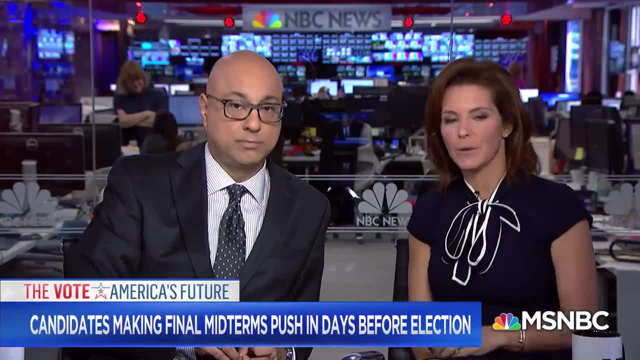 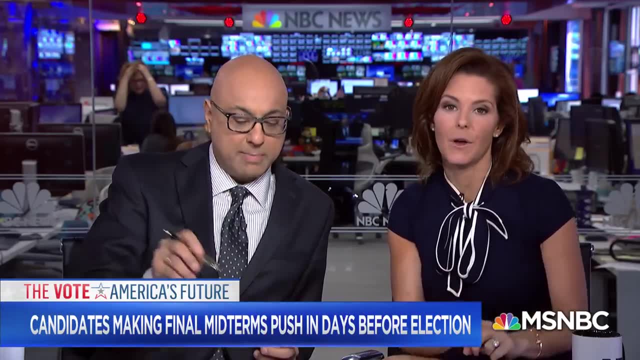 It will affect. It will affect almost no one watching right now. No one sitting here's lives, But health care, jobs, the economy, education. that's going to affect us all, Actually many of those types of people who come in seeking asylum or, in some cases, asking for it. 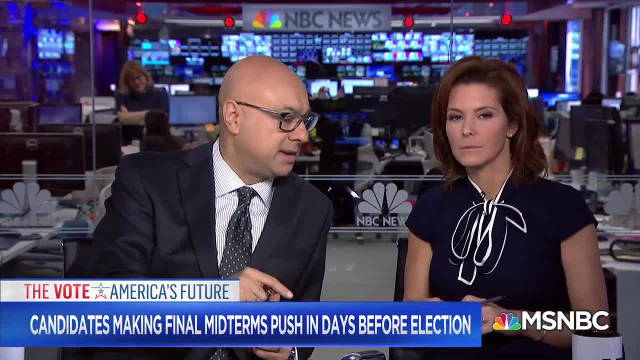 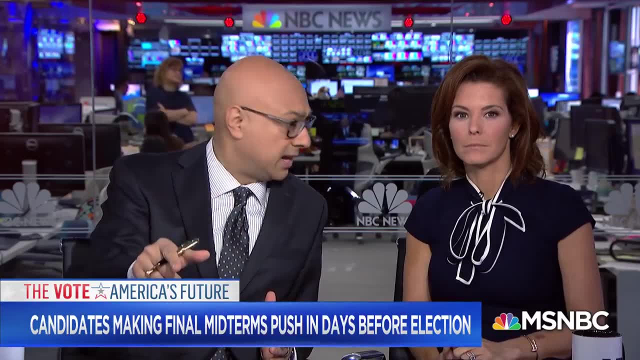 most of these people have to be asylum seekers. if they get work in the United States, It tends to be in minimum wage, service jobs or agricultural jobs. So in fact it generally only affects people positively from an economic perspective, because there are farmers across America. 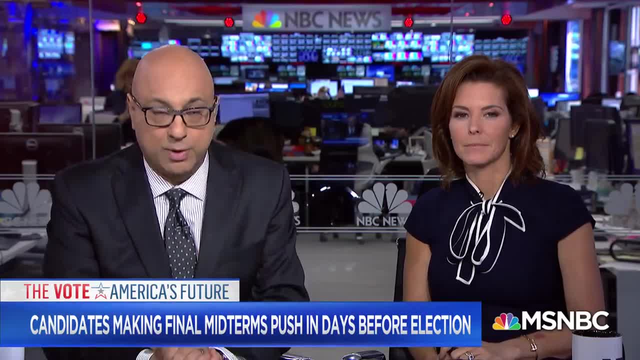 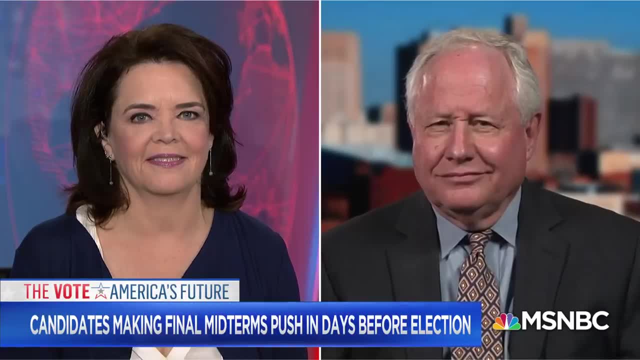 This is causing labor problems. Look, lots to discuss. So we brought Beth Foey in, senior editor of politics for NBC News, and Bill Kristol, editor-at-large of the conservative magazine, The Weekly Standard. Thanks to both of you for being here. 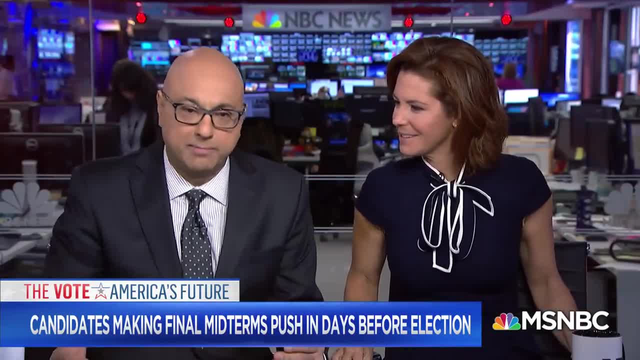 Hey, I just want to ask this one question. There are NBC Really Just one, Just one, And then you've got the rest of the show. Uh-oh, You've got 55 minutes left. You better think of some more. 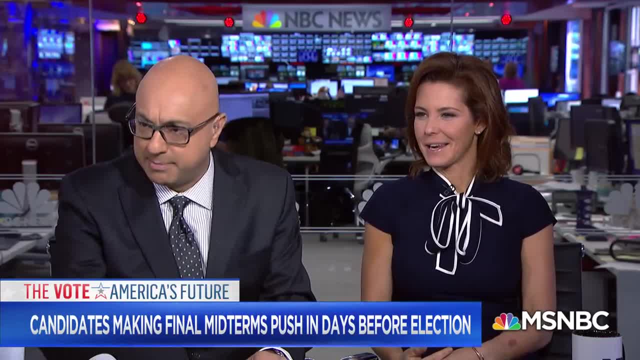 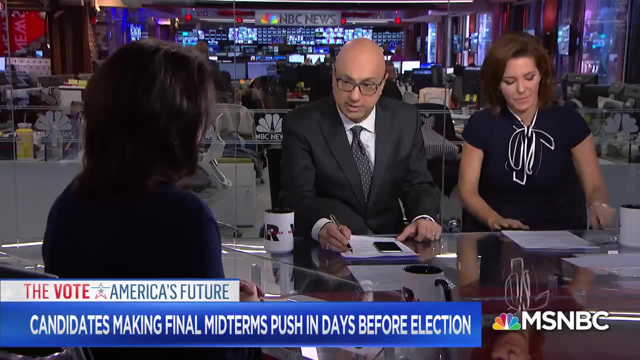 There are 11 seats in the Senate that NBC says are competitive. Of those three, Texas is an important one. Ted Cruz continues to have a lead and Republicans tend to be voting in larger numbers than Democrats. North Dakota- Heidi Heitkamp's at a disadvantage there. 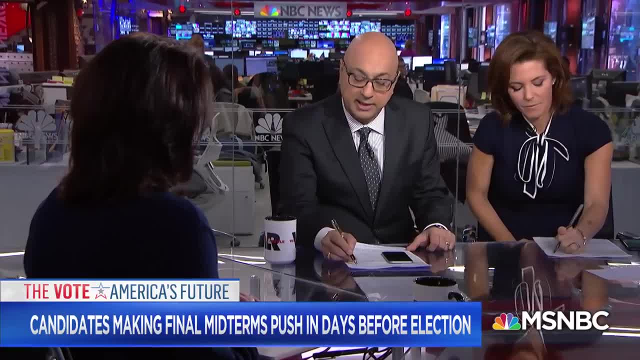 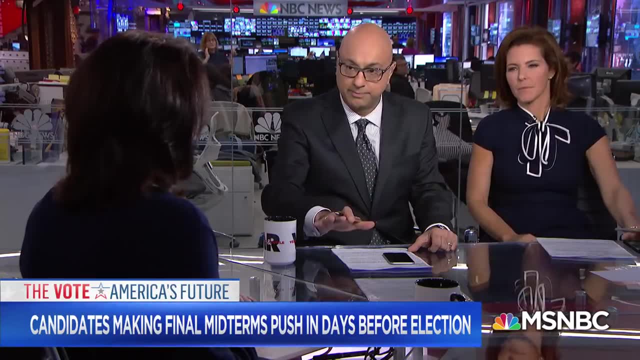 And Montana, where the president is going to be is. Claire McCaskill is in a very, very tight race there. All the Republicans need is three seats in the Senate to maintain control. Well, it depends. I mean, they've got control now. 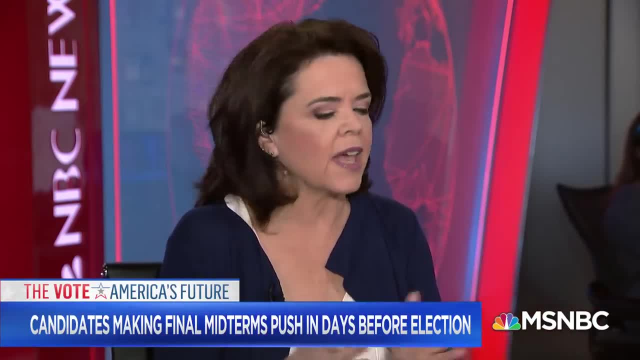 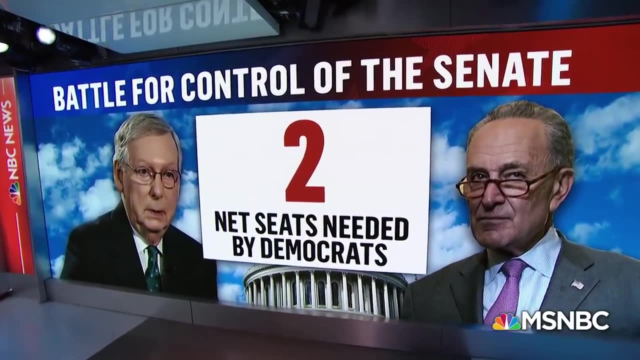 If things just stay the way they are, they're going to continue to have control. There's any way that you could slice this out. It could be a pickup of a couple of seats for Republicans. There is a path, As you said in your intro, for Democrats to take it. 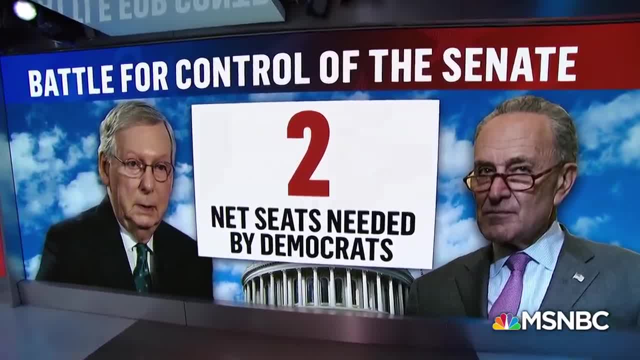 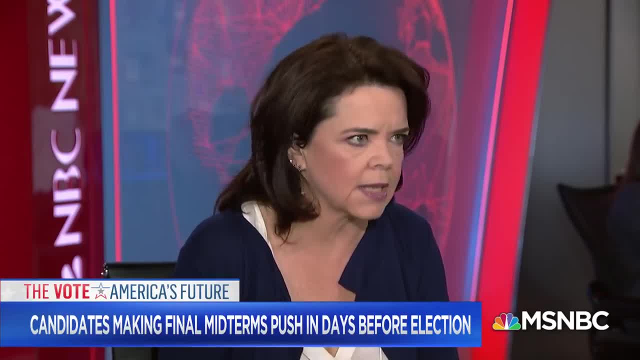 it would have to be a complete. It's narrow, but it exists. It would require- almost require- Heidi Heitkamp to win that seat in North Dakota, And polling shows her quite far behind now. The Missouri seat, the Indiana seat: really, really tight. 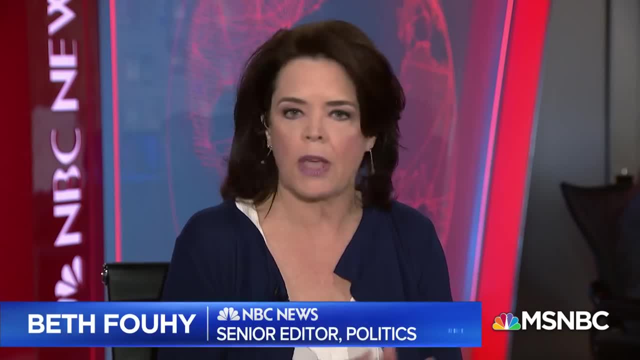 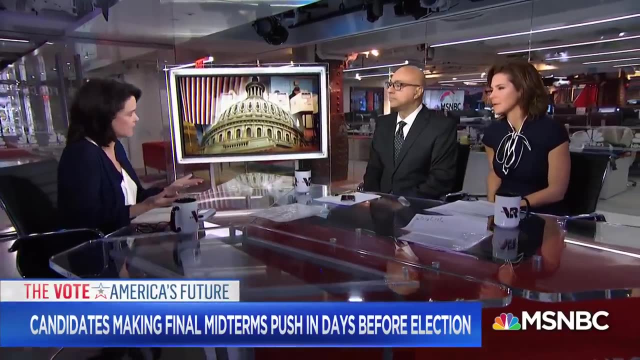 Montana. all those seats are red states held by Democrats. They were at a disadvantage right from the beginning because President Trump is so popular in those places. But all of those candidates- they're incumbents number one, so there's an advantage to incumbency. 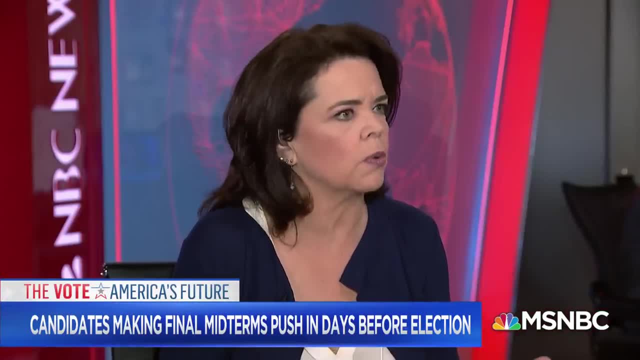 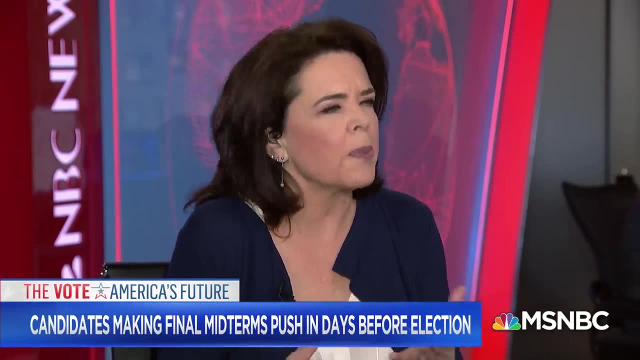 And all of them are pretty good representatives. They're not some sort of weird outlier that never should have been there. They're all from those states and they've got a long history in those states, So they're about the best people to be running in those tough red states. 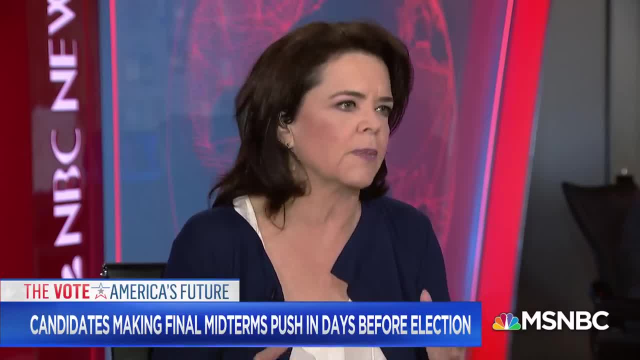 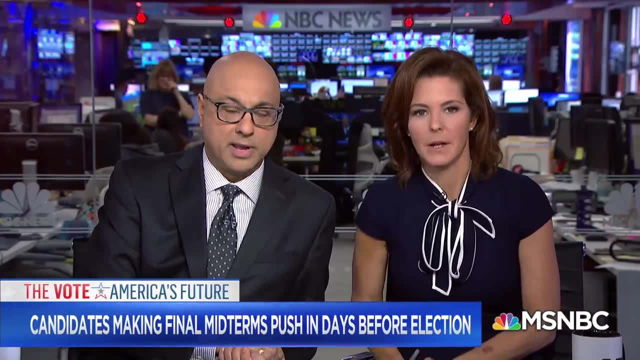 It's still going to be hard just because of the way that the map is looking for Democrats to pull off that inside straight, Friendly and loving way. You meant Missouri, not Montana, for Claire McKenzie. Absolutely, I meant Missouri. Thank you for correcting that. 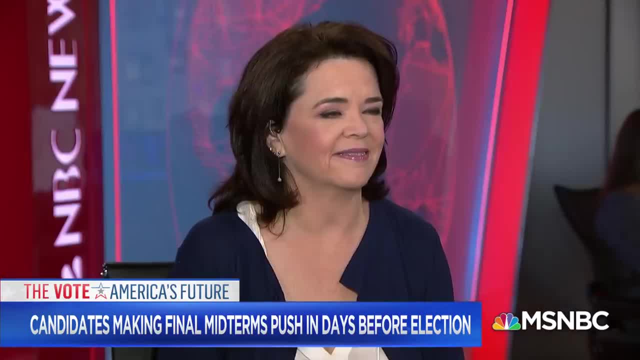 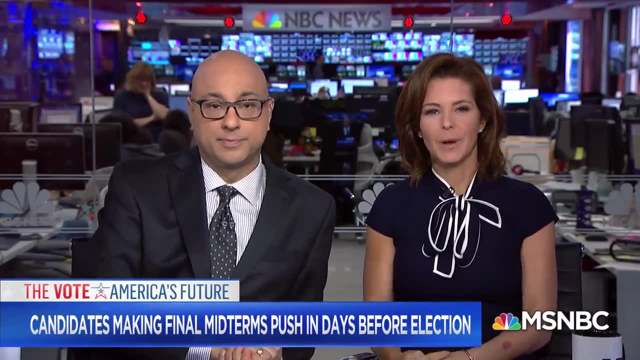 He's going to Montana too, Right, that's why I was confusing them, because the president's going to a lot of places which need shoring up and he's trying to help those candidates. Thank you for correcting me, Bill. what Senate race, which one do you think is the most important? 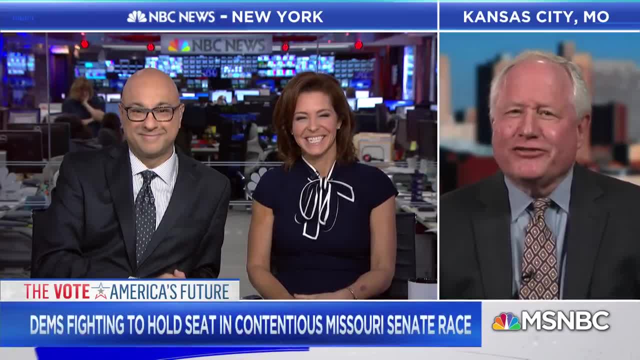 I'm actually here in Missouri, so I felt like I should say Missouri, which is a very interesting race, and I do think if Claire McCaskill doesn't win it it pretty much dooms Democrats' chances to hold the Senate. But look, there's still movement in this race. 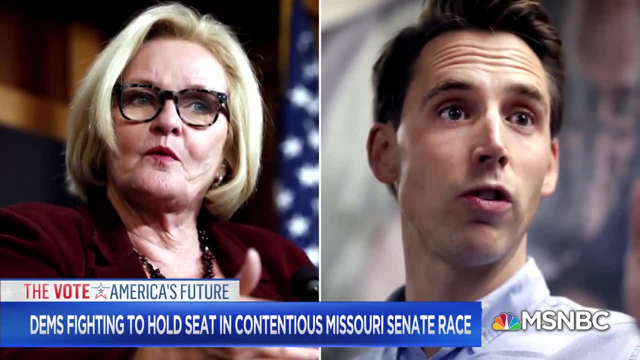 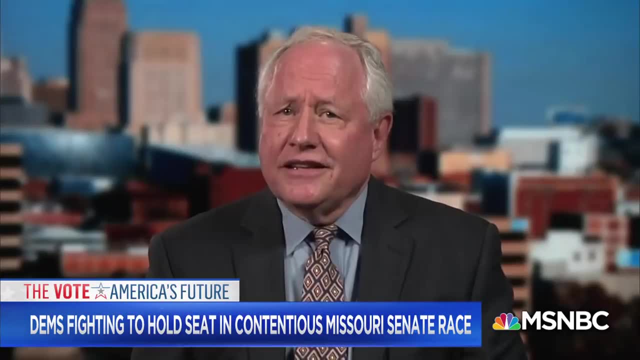 People are looking at polls. Today it's Thursday, That means they were in the field probably what Monday, Tuesday night? That's a week before the election. Most voters have made up their mind, but there are undecideds and they can break in one direction or another. 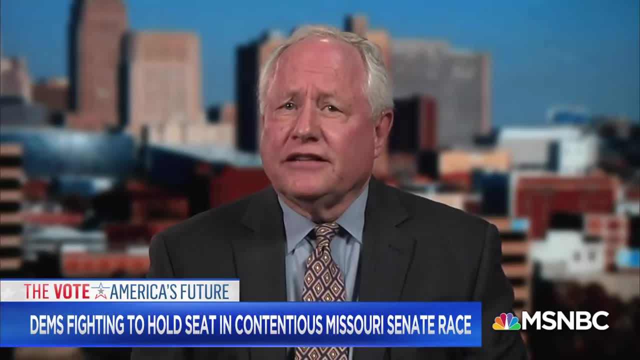 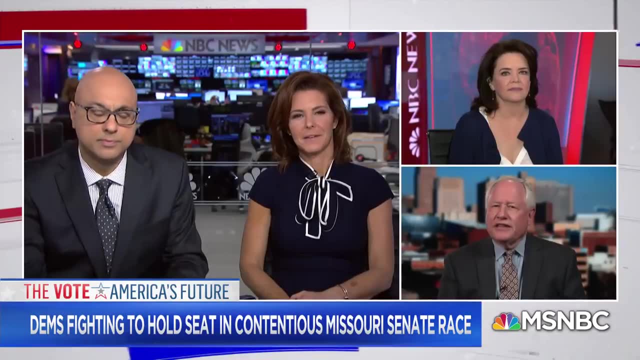 And then you get differential turnout. There are groups which can really affect an election And I'm a little less confident than everyone else that it's so impossible that the Democrats could win the Senate or that the House could go into a big Democratic number. 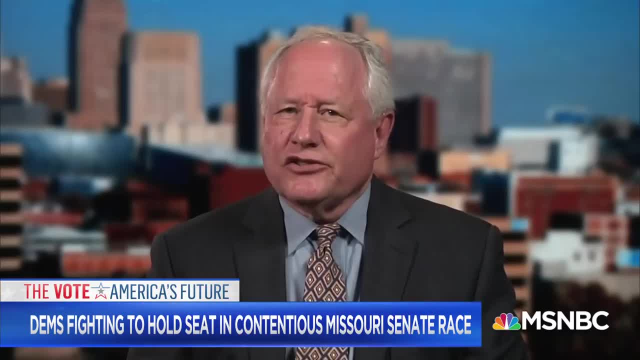 I just think I feel like there's a little momentum. Usually in these kinds of elections, when there's something of a wave, the wave recedes in early mid-October. There's kind of a bear market rally. I think we discussed this once before and you were amused by my use of the term. 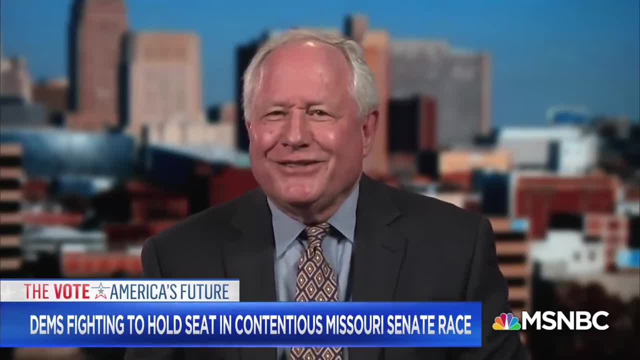 but I'm just, you know, trying to get our financial viewers interested here too, right, But then the major trend kind of reasserts And I think feel like that's happening. You see that a little more in the House polling. 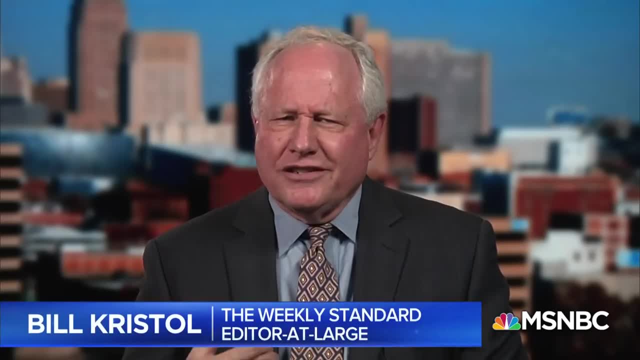 I just don't know. And so the one thing that Trump has done now is introduced immigration in such an incredible way, in a really, to my view, distasteful and dangerous way, But anyway into the race. I wonder how much that shakes things up. 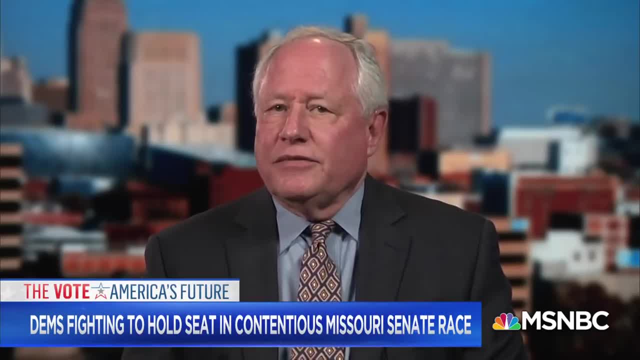 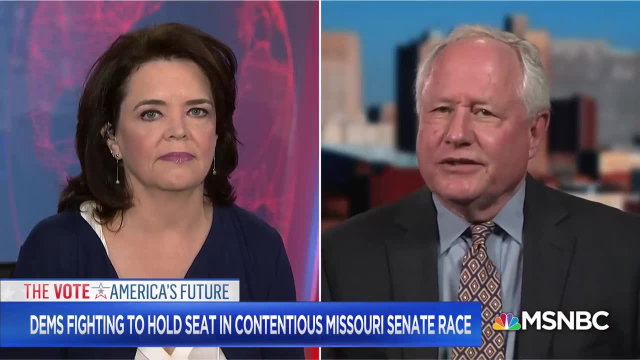 I think if I were a Republican candidate in some of these red states that Beth mentioned- North Dakota, even Missouri- I might just want a kind of a stable race where you say: you know what, we're the conservatives, they're the liberals. 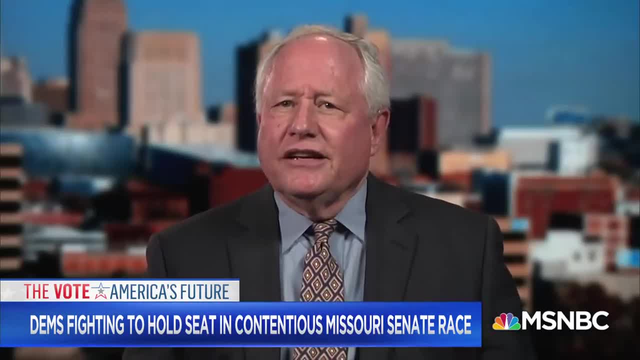 just let's have a normal election, so to speak. Indiana, Missouri, you know, and those go Republican obviously mostly. Instead they've got to. he's introduced something that his base loves, but I've got to think there are swing voters here in Kansas City, Missouri suburbs. 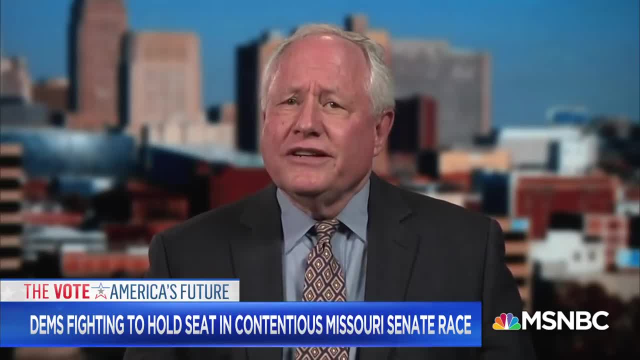 and the St Louis suburbs who look at that and think, geez, are we going to reward this kind of really extraordinary nativism and rabble-rousing? So I actually think Trump has put the Republicans at a little more risk by what he's done over the last two, three days. 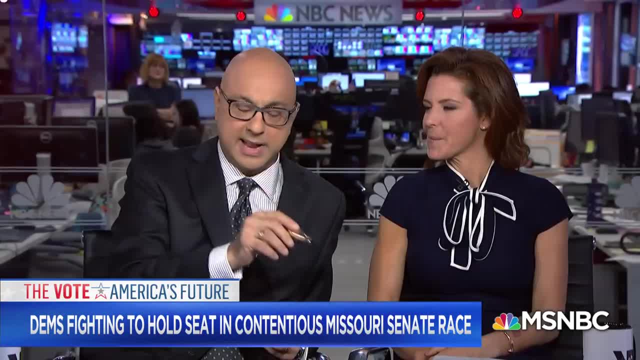 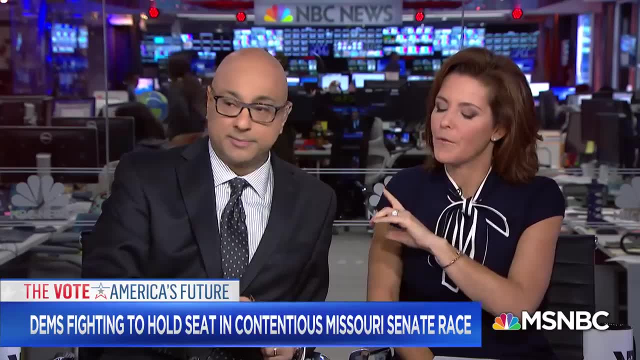 We've actually talked to a lot of Republican members of Congress from Kansas, Indiana, Missouri, Missouri, Iowa, Illinois, who all say we're not on side with this immigration thing. To that point, though, for those who are not on side, let's say those swing voters. 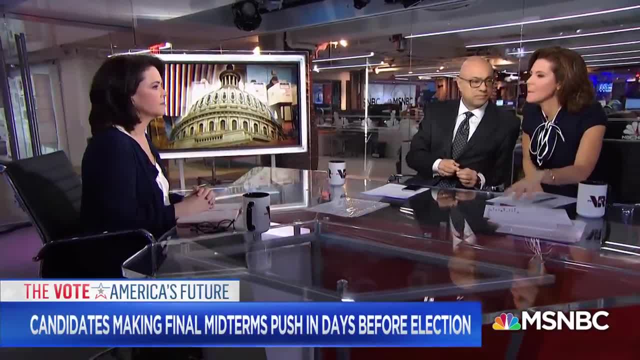 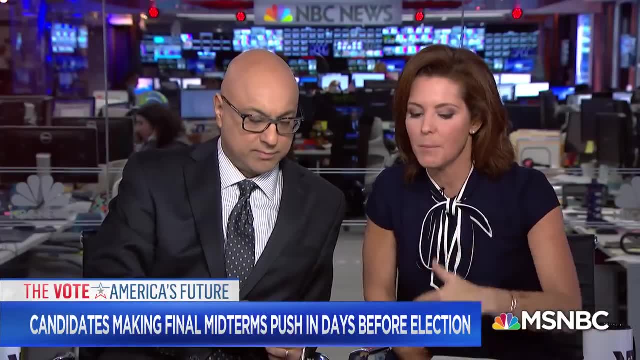 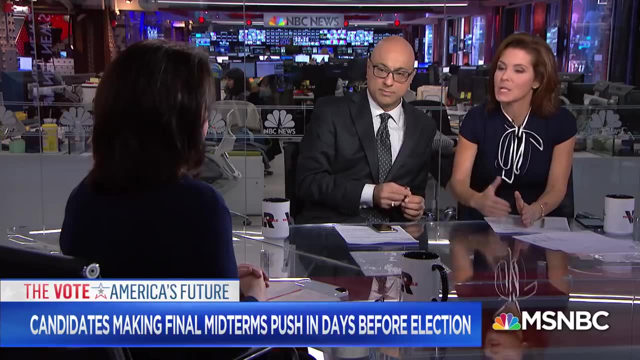 doesn't it matter who those Republicans are running against, Because if there's a swing voter that thinks the president's nativism approach, he behaves in a morally reprehensible way. those who think that's too much the chance they're a swing voter, and if their option on the other side is a far-left progressive Democrat. 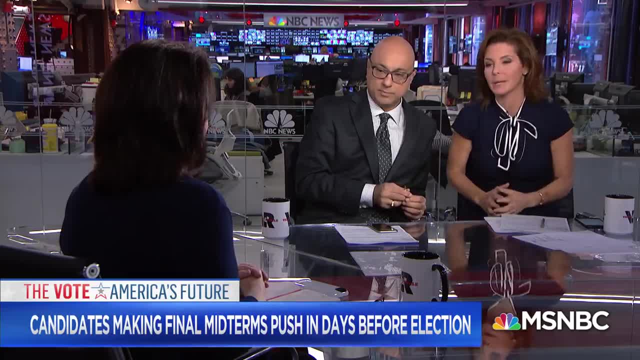 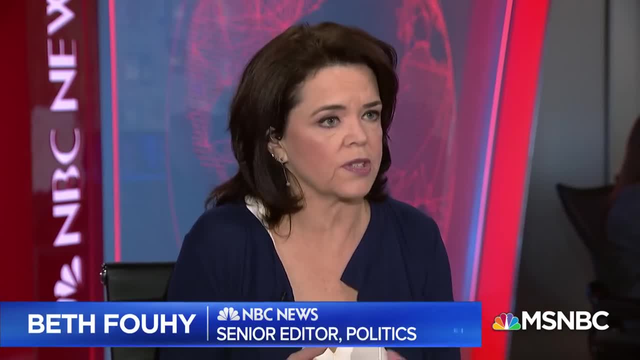 they've got a good chance. they're going to close their eyes, hold their nose and vote Republican again. Sure, it's possible, but what we've said all along- and it's becoming even more so the case now- is that this race is going to be all the races across the country this midterm. 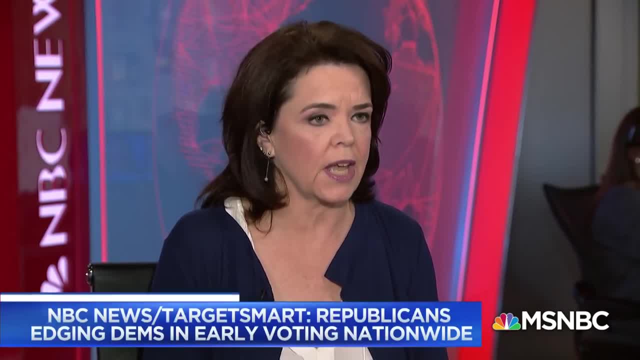 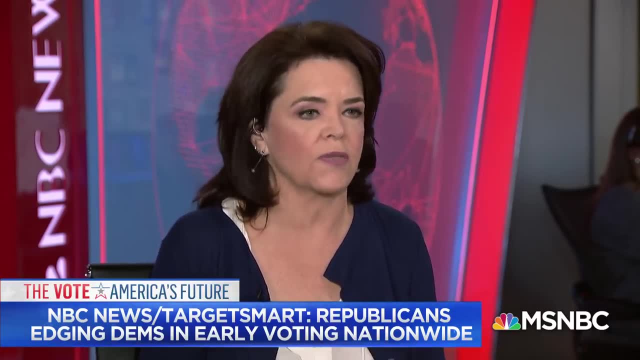 is going to be decided in the suburbs. Suburban voters are really, really engaged. they're really fired up, particularly suburban women. They're voting in. they're doing early voting in vast numbers. they've been the source of activism all of this time. 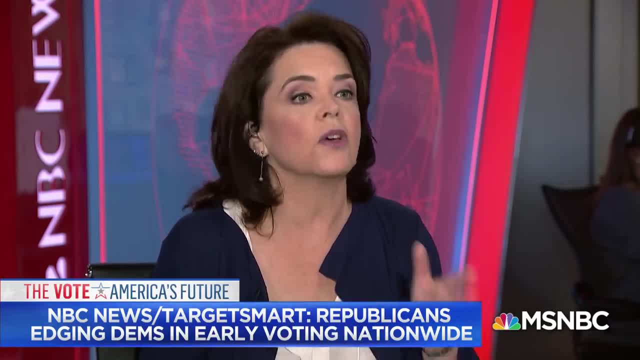 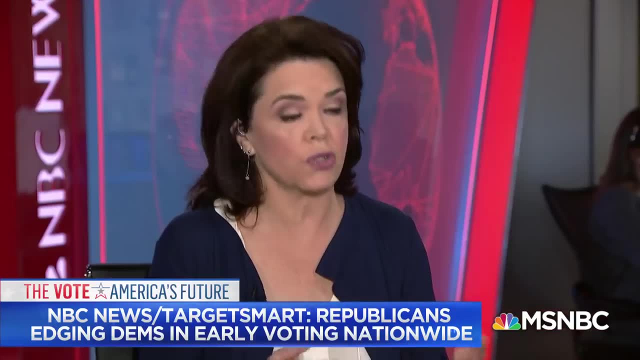 and they are going to be the voters who are the most important ones in this race. But in which direction? How is the immigration push that President Trump is now doing going to play in those suburban areas, which are typically very swingy? they tend to be very much mixed Republican and Democrat. 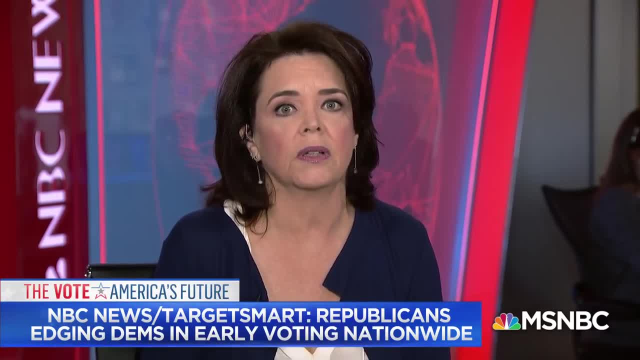 Bill says he thinks it's probably going to turn them off. Yeah, go ahead, Bill. Yeah, no, I just was going to say that I think, by definition, these Democratic senators in red states have won in red states, right. 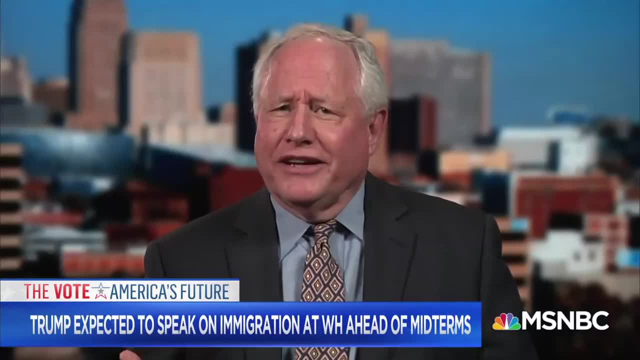 Claire McCaskill and Heidi Heitkamp, and so forth. so they're not left-wing. they're not. if you're a swing voter, you're not incapable, let's say, of deciding to come back to vote for them at the end. 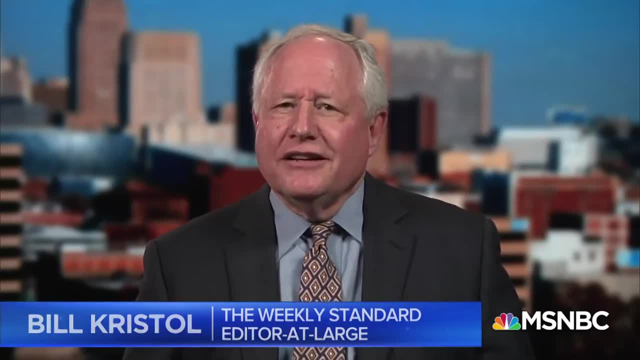 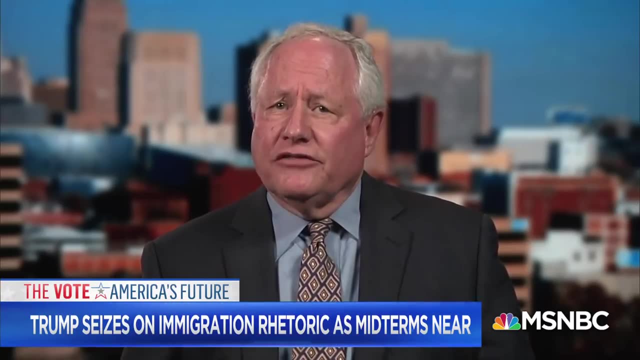 The other thing is it's very hard to judge for early voting. this is a famous trap that people get into. Having said all that, if we really are seeing a surge in early voting and if there's some surge in young people voting, if some of that is being captured- 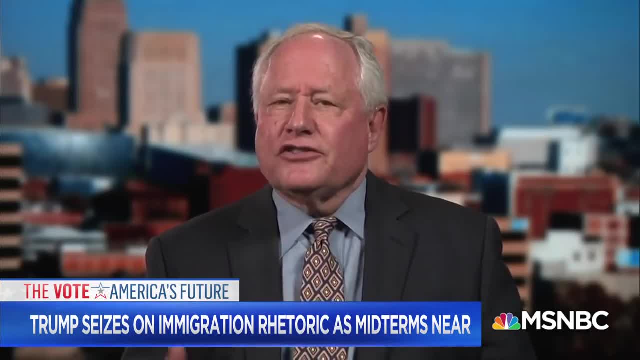 and if that. but more importantly, young people tend not to vote early, so if they vote on election day, that really changes things. I've looked. I'm sure Beth's done this. I've looked at some of these models a little more closely.